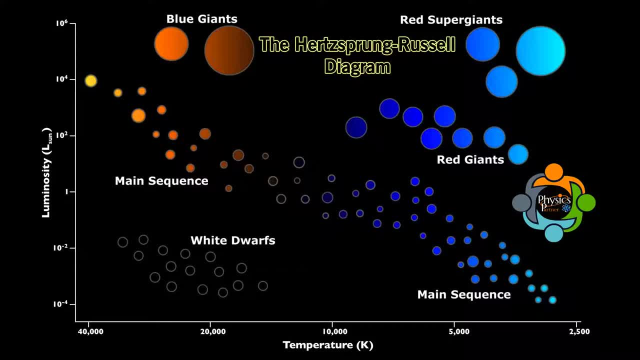 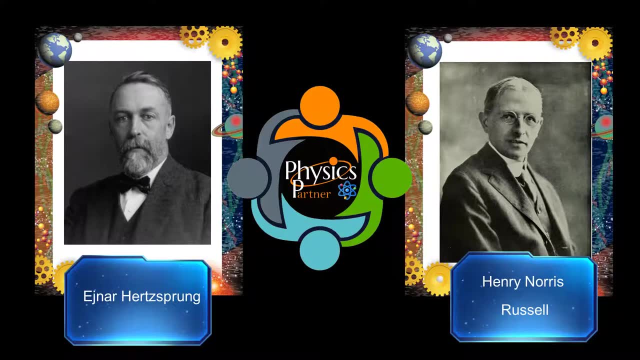 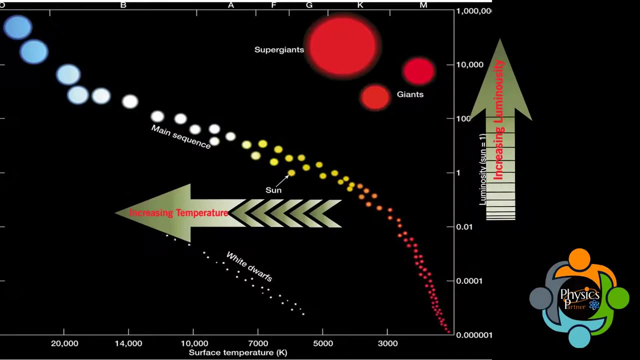 which is known as HR diagram, is one of the most important tools in the study of stellar evaluation. Founded independently in early 1900 by Eugener Hertzsprung and Henry Norris Russell, it plots the temperature of stars against their luminosity. I am talking about the theoretical HR diagram. 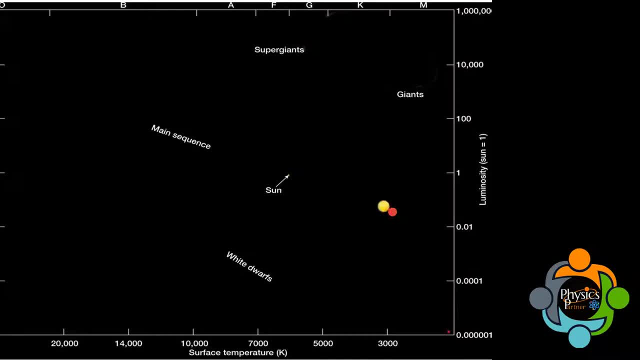 Depending on its initial mass, every star goes through specific evolutionary stages, dictated by its internal structure and how it produces energy. Each of these stages corresponds to a change in the temperature and luminosity of the star, which can be seen to move in the different regions of the HR diagram as it evolves. This reveals the true power of 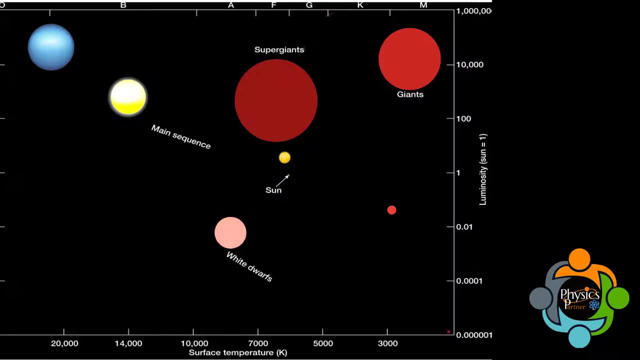 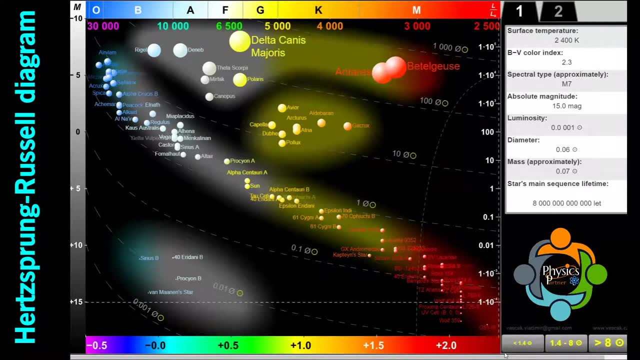 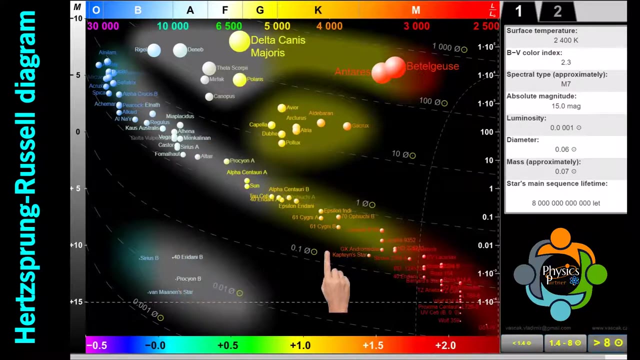 the HR diagram. Astronomers can know a star's internal structure evolutionary stage simply by determining its position in the diagram. Let's do an interactive activity about the HR diagram. This HR diagram on your screen shows a group of stars in various stages of their evolution, By far the most prominent. 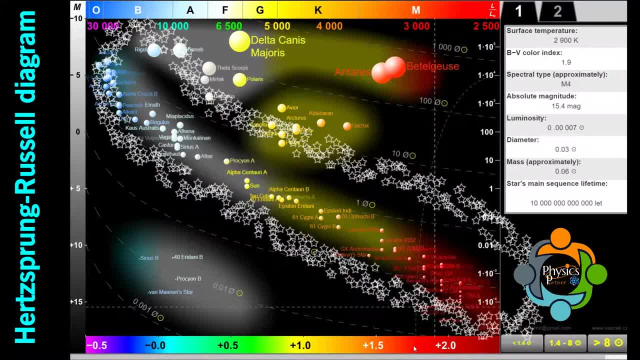 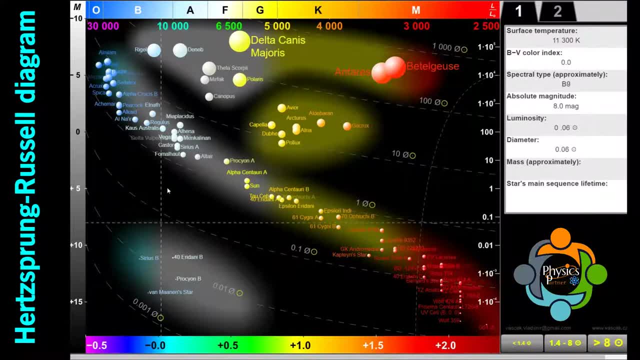 features in the main sequence which runs from the upper left- you can see here hot, luminous stars- to the bottom right, which is cool and faint stars of the diagram. The giant branch is also well populated and there are many white dwarfs You can see here there. 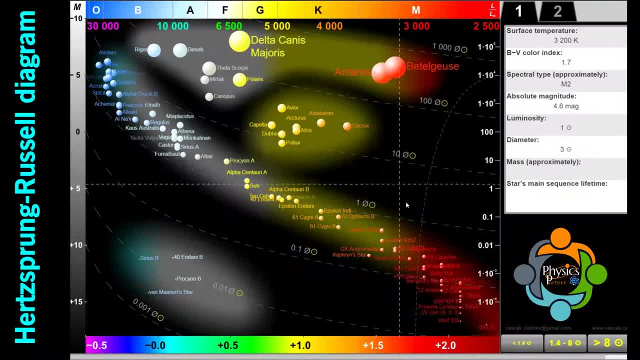 are three main regions of the HR diagram. The main sequence, which is absolutely the main one, is stretching from the upper left- hot, luminous stars- to the bottom right. cool, faint stars dominate the HR diagram. On the right of the screen you can see the changes. 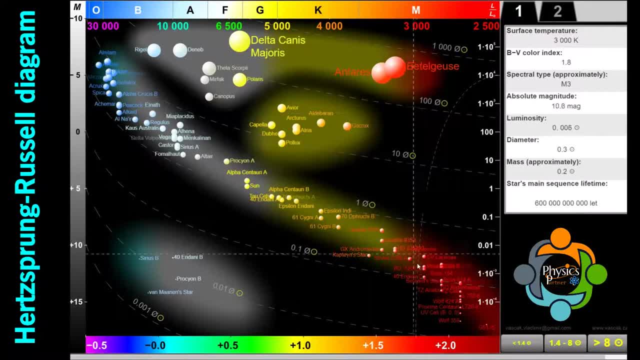 in the luminosity and temperature. It is here that stars spend about 90% of their lives burning hydrogen into helium in their cores. Main sequence stars have a Morgan-Kehner luminosity class labeled 5.. Number 2 region is a red giant and supergiant stars, which is considered as luminosity class. 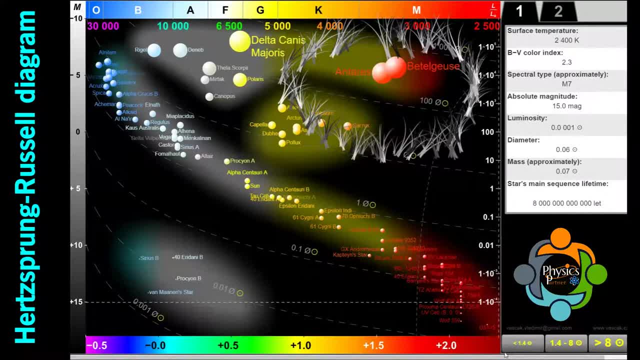 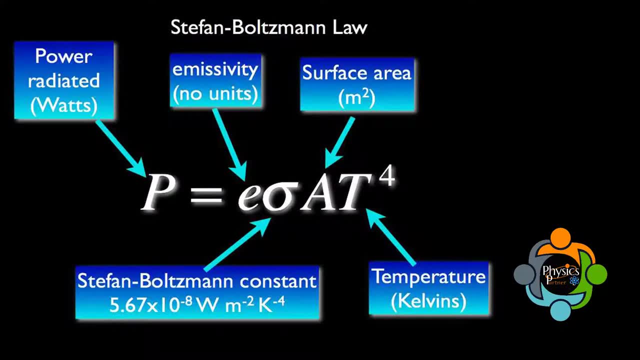 1 through class 3 occupy the region above the main sequence. They have low surface temperatures and high luminosities, which, according to Stephen Boltzmann's law, have a luminosity of about 1.5.. They have also large radii.